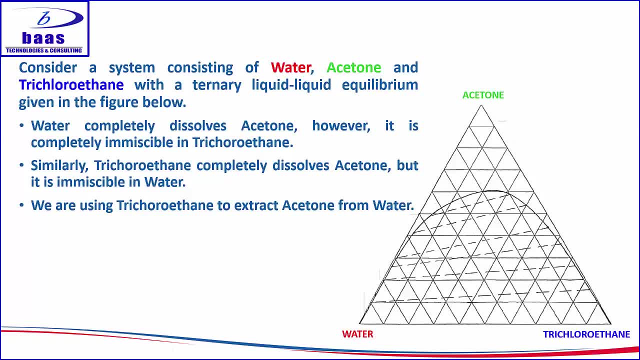 because the way our liquid-liquid phase is split is: you will have a phase with which you have water and acetone, and then a phase with trichloroethane and acetone. As you continue with this lesson, you will understand why I am saying that water completely dissolves. 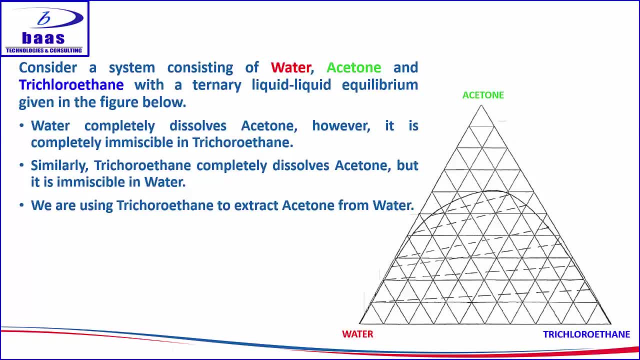 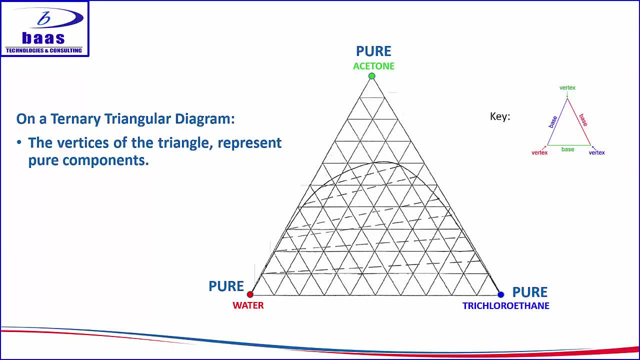 acetone and trichloroethane completely dissolves acetone. However, water and trichloroethane are completely immiscible. Let us just take a few minutes to unpack how the ternary triangular diagram works, Keeping the terminology. if you look at the triangle key in the corner- here the corners- 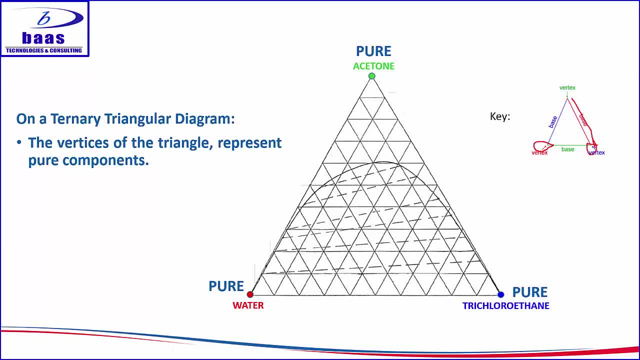 will be the vertices, and then the sides will be termed the bases. If you look at the vertices of our triangular diagram, you will notice that the vertices represent pure components. Here you have pure acetone, pure water and pure trichloroethane. 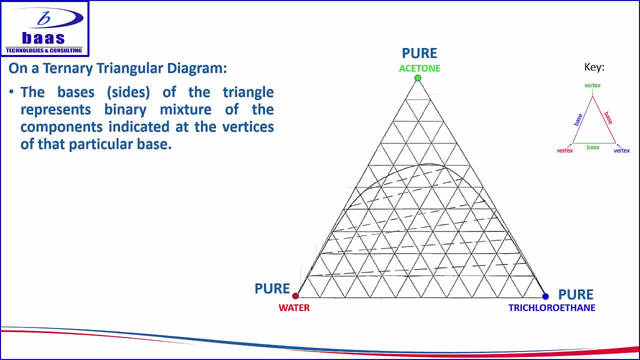 The bases or the sides of the triangles represent binary mixtures of the components indicated at the vertices of the particular base. What essentially this is saying is: this base represents a water-acetone binary mixture. This base represents acetone-trichloroethane. 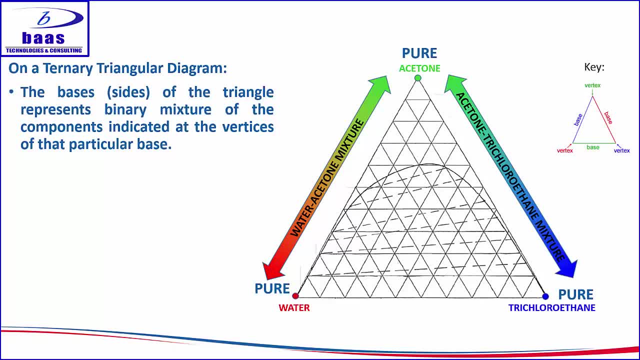 mixture at the vertices, and this is what we are talking about here. This is a combination on that particular base- acetone and trichloroethane- and then this base represents water and had trichloroethane mixture. the bases also represent zero. 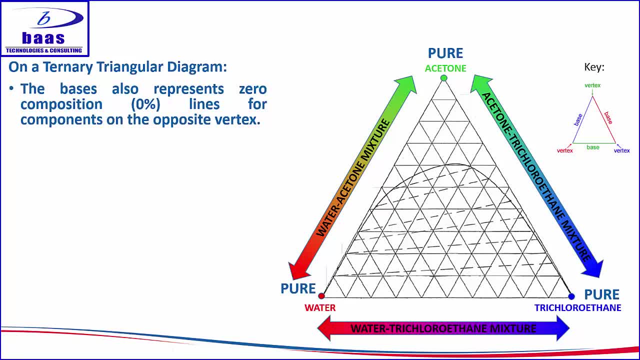 composition lines for the component on the opposite vertex of that base. what we are saying here is a, this vertex, which is a. so this base, which is a acetone water binary mixture, represents a zero percent composition line for trichloroethane, which is on the opposite vertex of the space, as you go across. 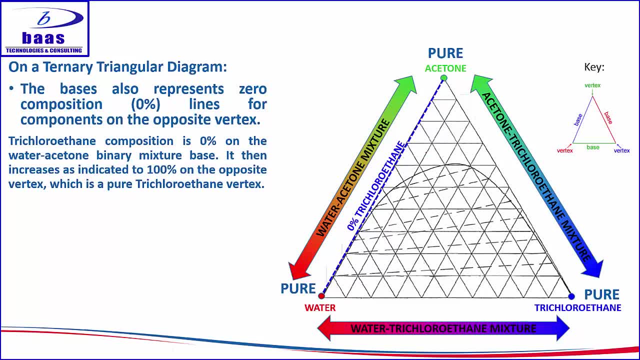 with the base parallel going towards the vertex, the composition of tri-chloroethane increases from 0, 10%, 50%, 80% all the way to 100% at the vertex. On the side of the acetone tri-chloroethane, you have the 0% water line, as water is on the 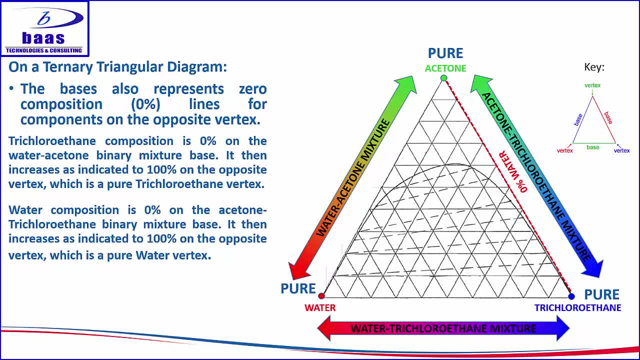 opposite vertex of this base and the composition of water here is 0 and it increases along as you move towards the vertex. Similarly, for acetone, on this binary water tri-chloroethane base, you have a 0 acetone composition line and the composition of acetone increases as you move. 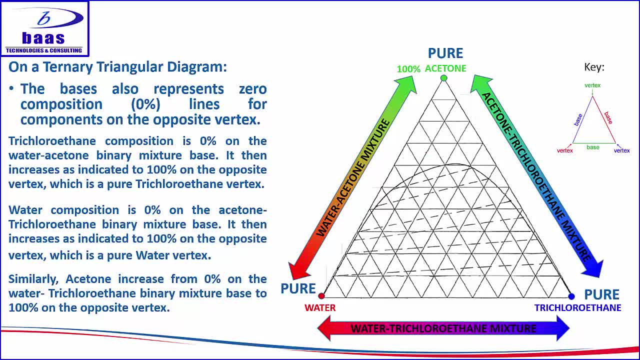 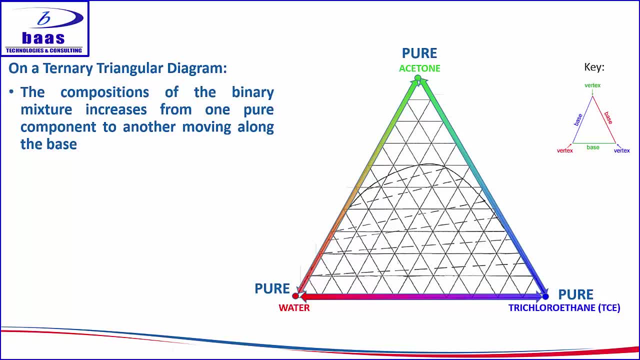 towards the pure component vertex of acetone. The compositions of the binary mixtures increases from one pure component to the other as you move along the base of the triangle. If you look at the water acetone mixture, the composition of the tri-chloroethane line increases along the 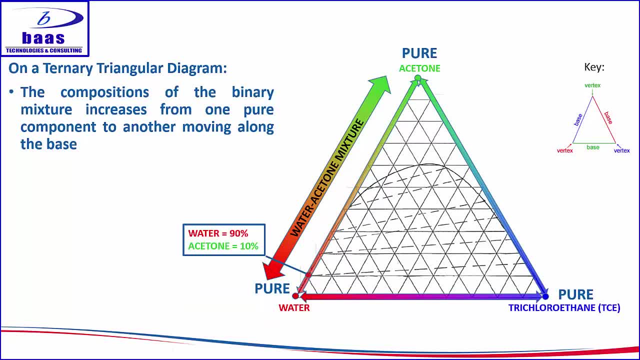 transition starts from the pure water vertex and it increases as you move along that base, increasing the composition of acetone and reducing the composition of water, moving all the way to the pure acetone vertex. Similarly, if you look at the acetone tri-chloroethane mixture, 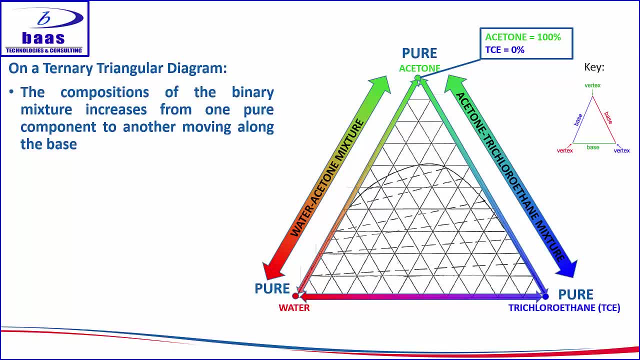 the composition increases from 0 and 100%. it changes from that all the way towards a pure trichloroethane composition and similarly for the water trichloroethane mixture you will have on the trichloroethane vertex you will have. 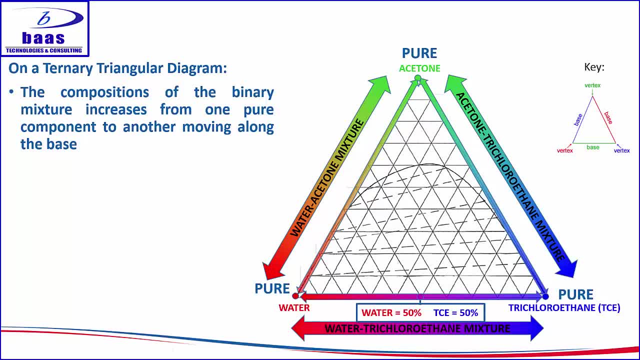 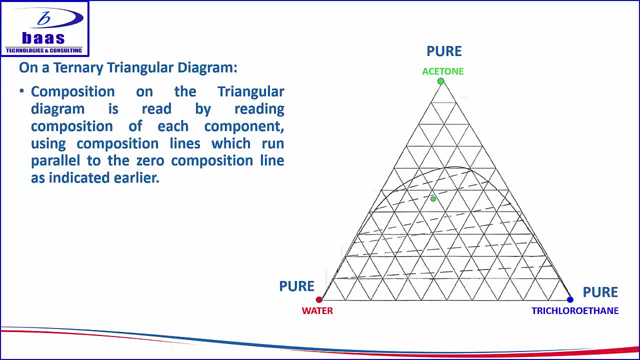 100% trichloroethane and 0% water, and then the composition of water increases as that of trichloroethane decreases, moving from the pure trichloroethane vertex all the way to the pure water vertex, The composition. 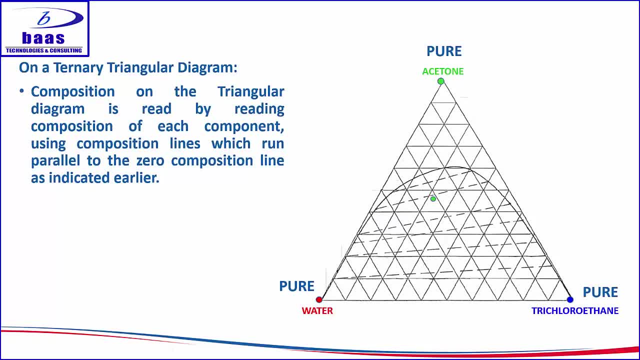 on. a ternary diagram is read by reading: composition of each component using the composition lines which run parallel to the composition lines. as we have indicated earlier on, Composition of water will start being zero here and then the composition will increase. If you want to read a composition of water, 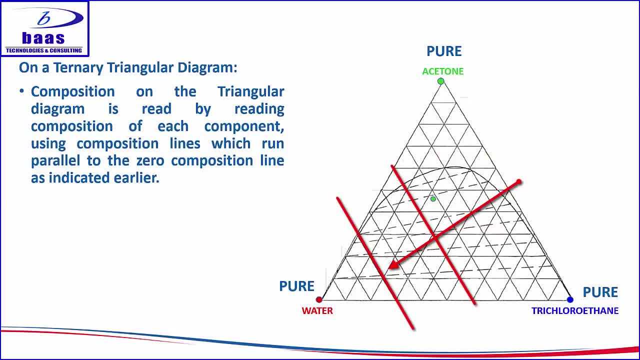 at any point, you will use a composition lines that run parallel to the zero composition line of water. Let us exemplify that with a point indicated on the map. The composition of acetone at this point can be read using the lines that are parallel to the zero percent composition for acetone, which is the 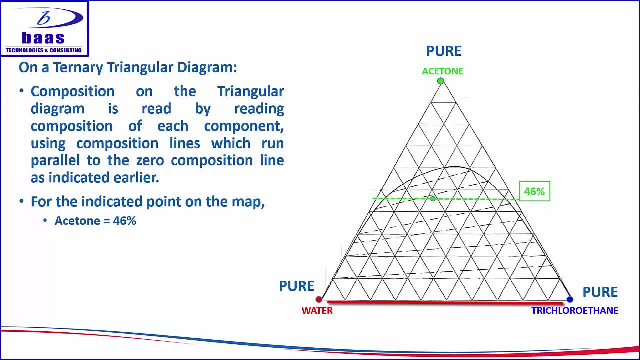 line here on the water trichloroethane binary mixture base. So if you look at this, you have 0% acetone, 10% acetone, 20%, 30%, 40% and somewhere there you have 46% acetone. 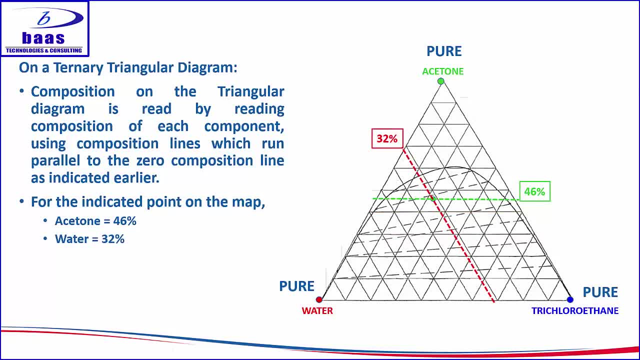 For water. similarly you can start this way: 100% water, 90,, 80,, 70,, 60,, 50,, 40 and somewhere there you have 80, and then this represents a 32% water line. and similarly for the trichloroethane line. We could have calculated the trichloroethane. 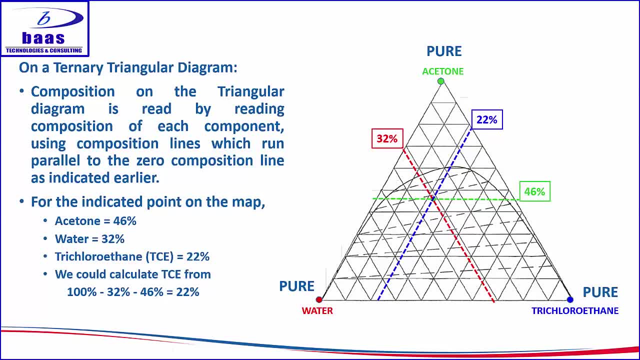 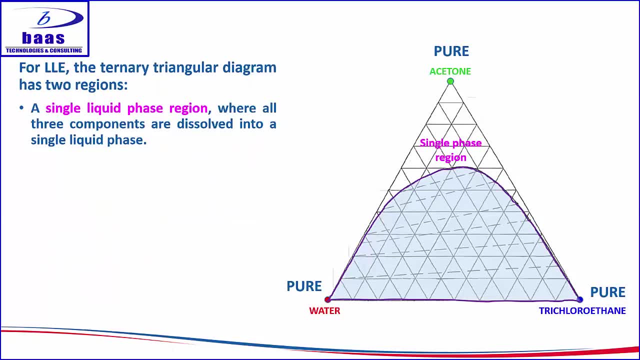 from just component balance, knowing that in a mixture the all of the three components have to add 200% Liquid. look at a ternary triangular diagram. We know that we have two regions where we have a single phase region where all the three components are miscible in one liquid phase, and then we have a two phase region where a 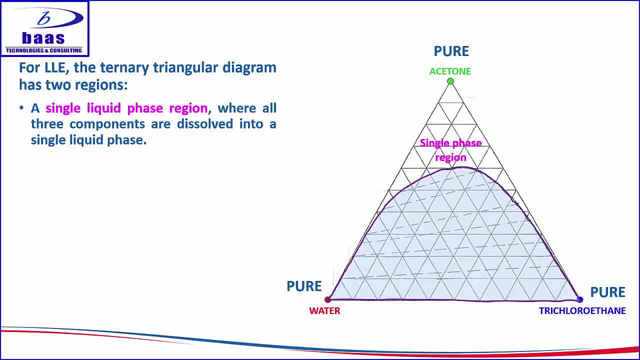 mixture in that region will split into two separate liquid phases. If you look at this acetone water trichloroethane system, here represents the single phase region and then in here you have your two liquid phases regions. the mixture in the composition space will split into two. 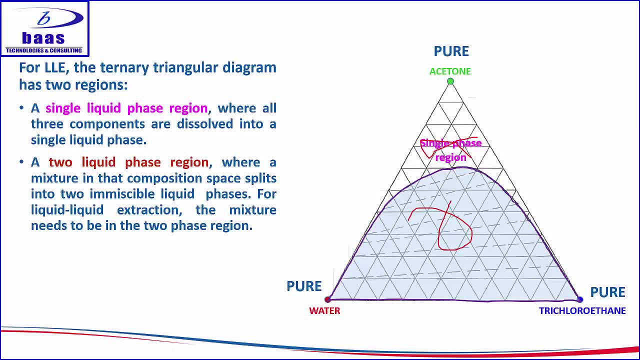 immiscible liquid phases. For llquid liquid extraction to occur, you need to be operating in the two mention. the two is the liquid phase. The two regions of immiscibilty are divided by the immiscibility boundary, which represents the liquid liquid equilibrium. with the, the two liquid phases. this is called liquid liquid equilibrium. within the two regions of immiscibility is the quarter liquid liquid. If we just want to use liquid liquid in both cases, do not use liquid liquid in both species because in this translation it will be missing between the two and sugar, Let me just�cektallyではah model, which represents the, the liquid liquid equilibrium within the uty and sur gaming distance of talked than in two regions And in thiscektally in trouble here we've really 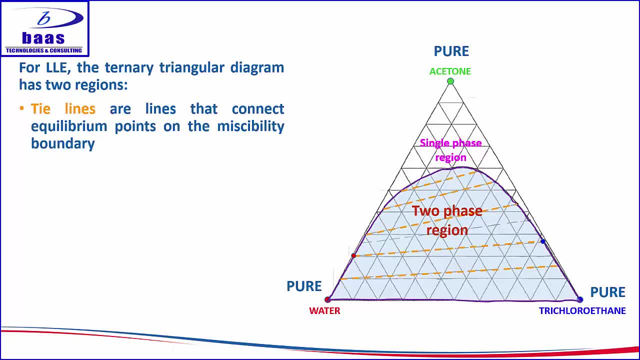 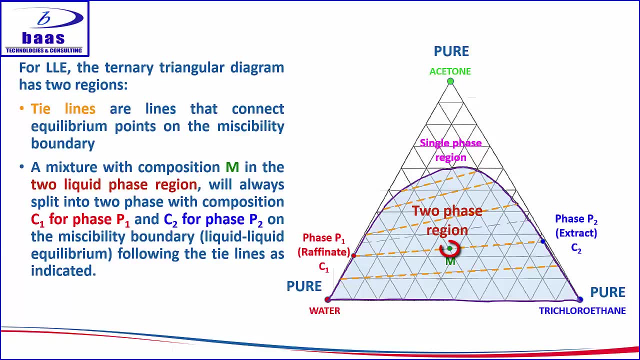 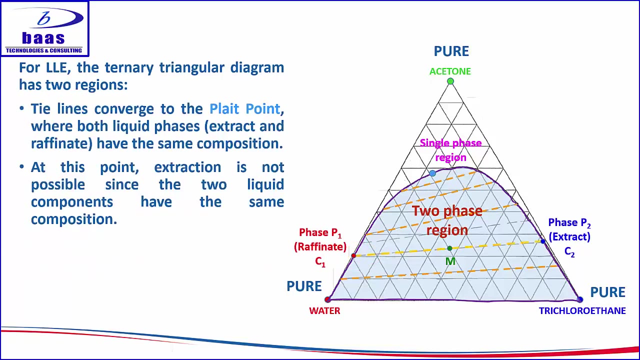 phase region, you have tie lines which connect the equilibrium points on the miscibility boundary. What this essentially means is that a mixture with composition M in the two liquid phase region will always split into two phases, with composition C1 for phase 1 and then composition C2 for phase 2.. We have 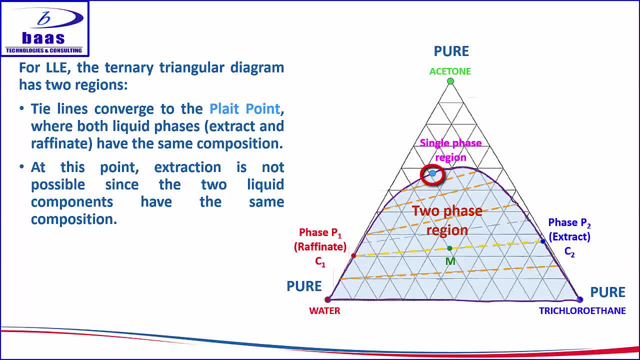 a point called the play point on the liquid-liquid equilibrium ternary diagram. If you look at the tie lines as you move from this all the way to the top, you get to a point where the tie lines disappear. At this point you 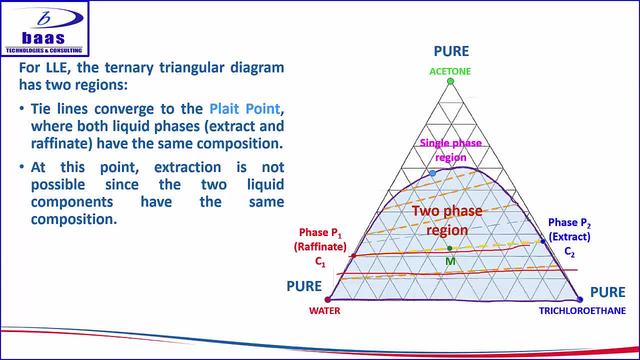 still have two liquid phases. However, the two phases that are split, they have the similar composition. If you could remember azootropes from VLE, So this is an azootrope for liquid-liquid equilibrium. We are going to be looking at an example where 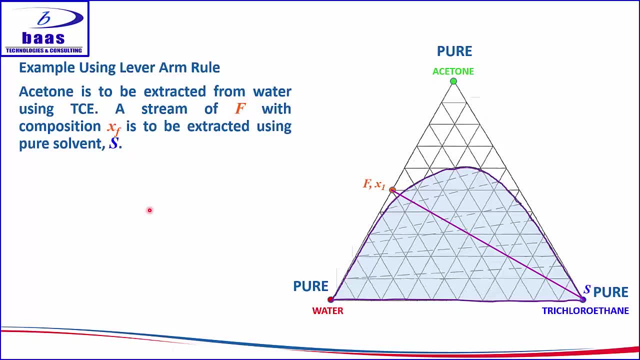 we are going to be extracting acetone from water using trichloroethane. Our feed will be termed F with composition XF, which is a binary mixture of water and acetone, As you can see, is located here on the binary mixture base of water and acetone, and then we will be extracting that with. 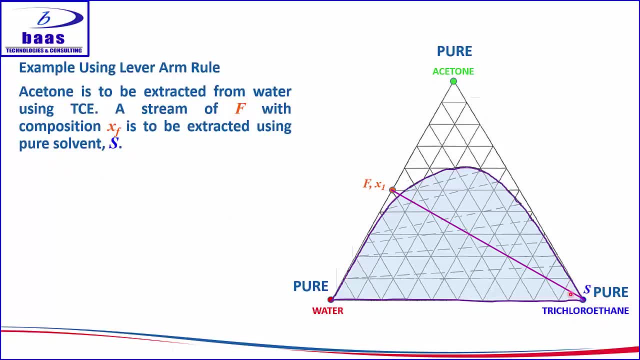 pure acetone solvent S, which is located at the trichloroethane vertex. here The points S and F on the triangular ternary diagram define the mixing line. The mixture point M locates the position of the two streams F and S after they've been. 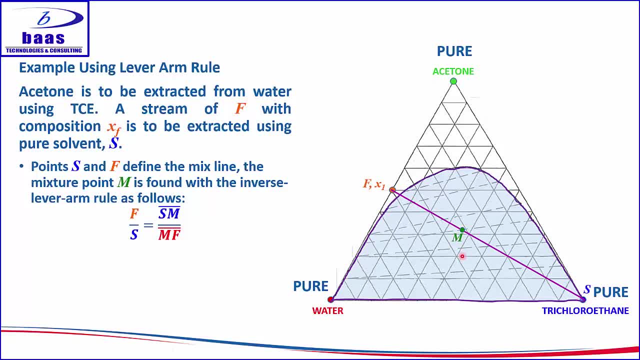 mixed. The location of point M on the ternary diagram can be located using the inverse lever arm rule. Please note the inverse lever arm rule how it applies. You have F, which is located here on this side, and then you have SM line, segment SM, which. 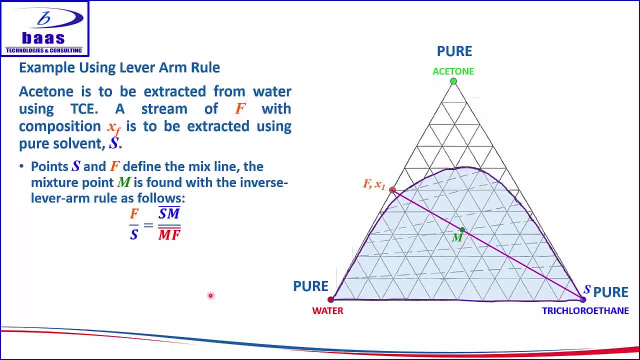 is located on the other side of F, and then you have S, which is the solvent, located here, and then you have line segment MF, which is located here on the opposite side, Just indicating that SM is located on the opposite of F, Okay, And then MF is located on the opposite side of S, and then SM and MF are line segments. 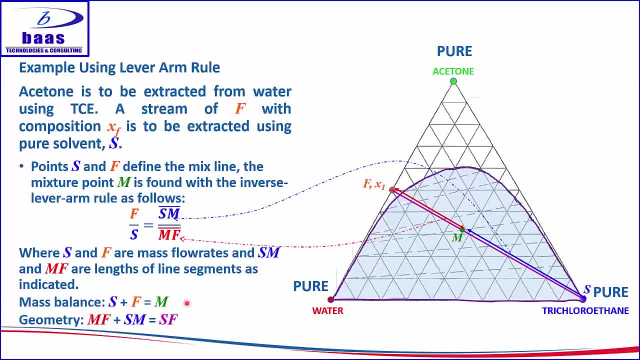 as indicated on the diagram. If you look at mass balance, M will be equivalent to S plus F, and then if you look at the geometry SF, the total length of the line segment is equal to the two shorter line segments combined. So line segment SF is equal to line segment SM. 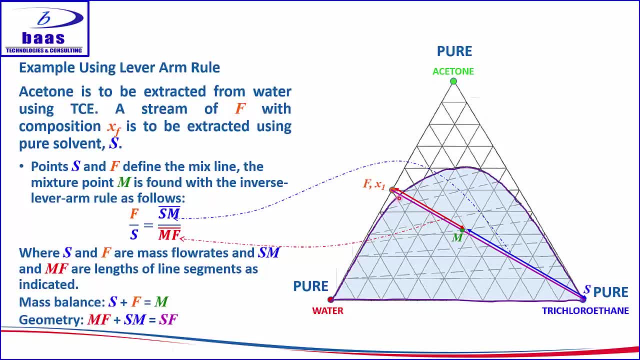 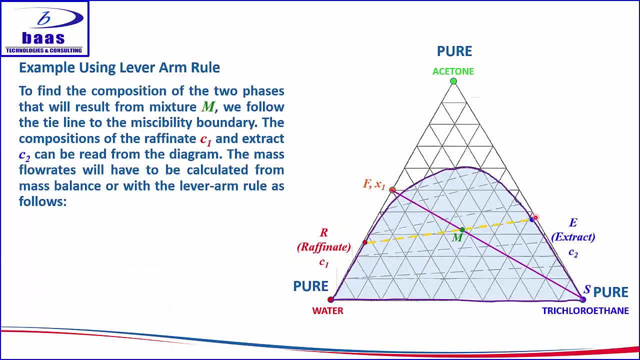 You have LL equals LL, and now you have FM equals LL, M is the maximum And MF is now equal to LL. Okay, now let me move onto the composite of the two phases, So 2 phases, And these two phases must be interchangeable because of the mass flow ratio, which we know is P1. 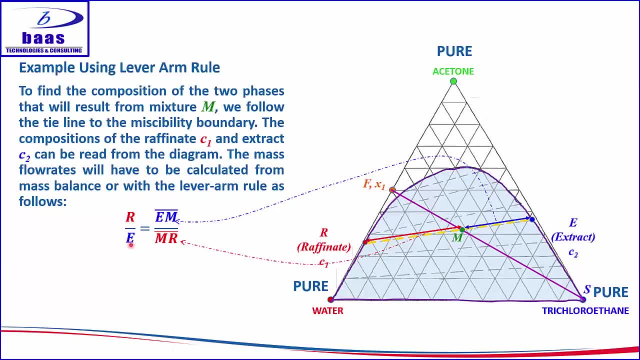 The mass flow rate of R over the mass flow rate of E is equal to line segment EM, which is this line segment, over line segment MR, which is this line segment. And then again, where E and R are mass or molar flow rates, if you look at mass balance, E plus R will be equal to M. 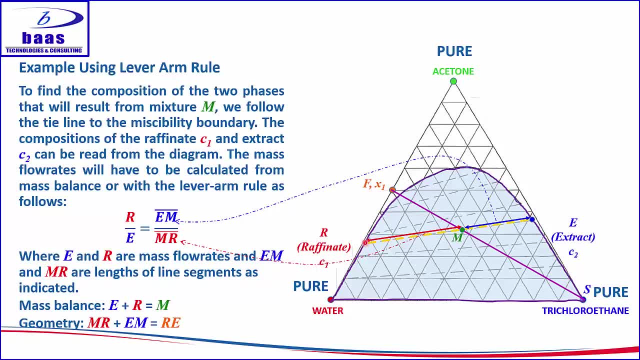 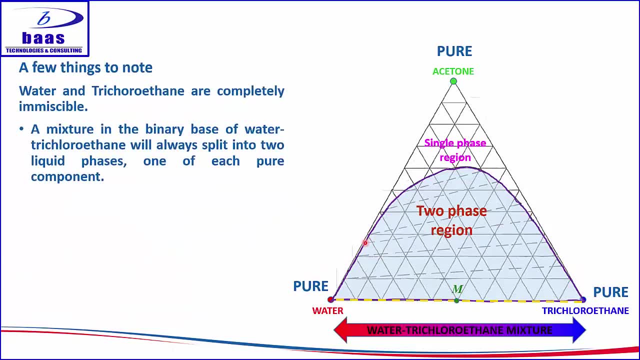 And then, if you look at the geometry, the length of line segment MR plus the length of segment EM will be equal to the length of the segment ER. Water and trichloroethane are completely immiscible. A mixture in the binary base of water and trichloroethane will always split into two liquid phases, one of each pure component. if you look at this, 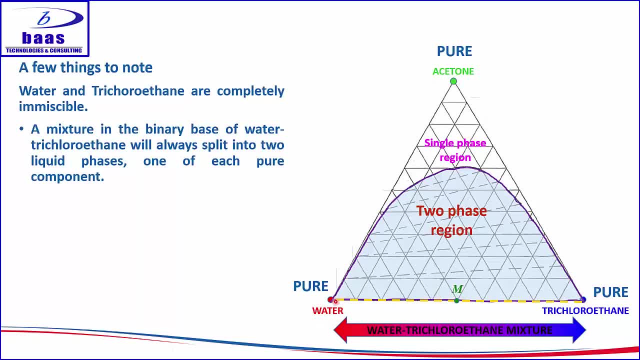 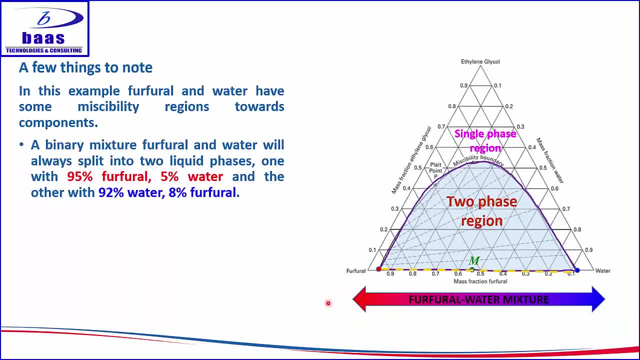 This is a two-phase region. Any mixture here will split into pure- So trichloroethane- and pure water. Let's look at an example that is different from what you have looked at. In this example, Pfefferal and water do seem to show miscibility towards pure component water or pure component Pfefferal. 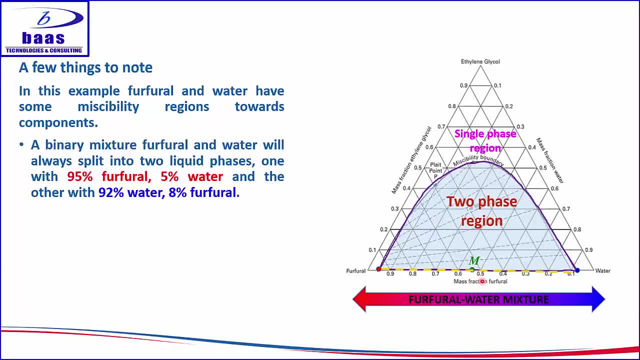 If you look at the binary mixture of Pfefferal and water, it will always split into two phases: that contains 95%, 5% Pfefferal, 5% water, and then the other that contains 92% water and 8% Pfefferal. 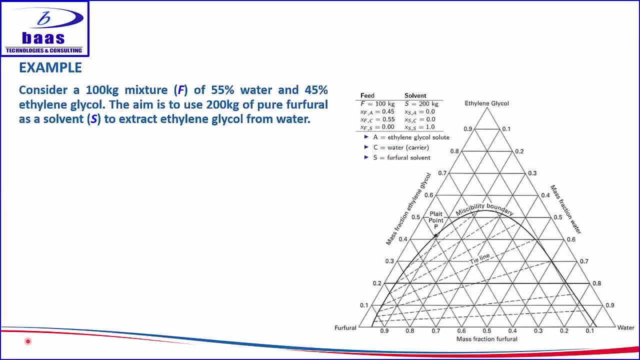 Let's conclude this lesson by looking at an example where we will do some calculations. Consider a mixture F of 100 kg of water and ethylene glycol. where you have 55% water and 45% ethylene glycol, The aim is to use a 200. 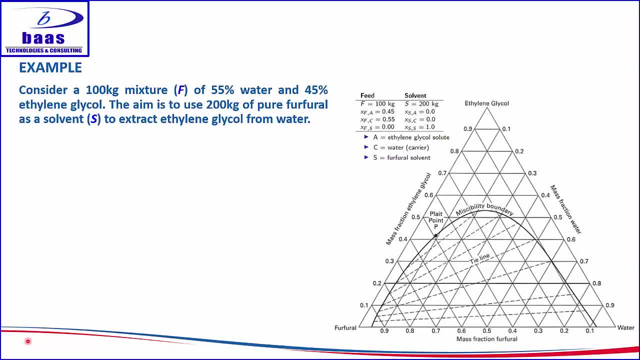 200 kg of pure solvent S, which is Pfefferal, to extract ethylene glycol from water. The mixture F is on the water-ethylene-glycol binary base as we have located it over here. Mixture F is on the water-ethylene-glycol binary base located here. 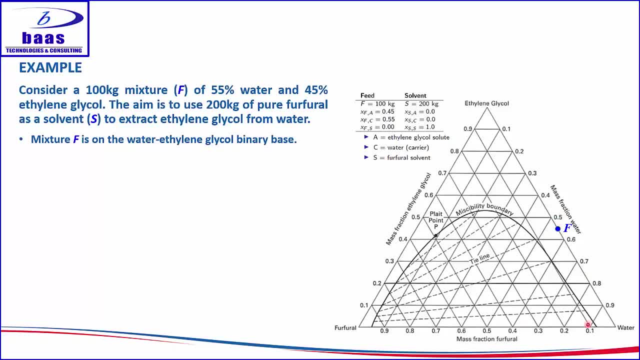 And if you look at it, we have a. if you look at the water, we have 55% on the spiral line And then, if you look at ethylene-glycol, we are on 45% on the line that will be running parallel here. 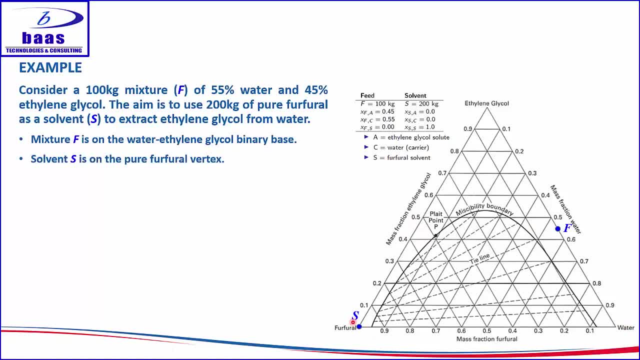 Solvent is pure. It's situated at the Pfefferal vertex. The resulting mixture, M, will lie anywhere on the line joining F and S. The position can be located using mass balance to calculate the composition of M, Because you know the specifications. 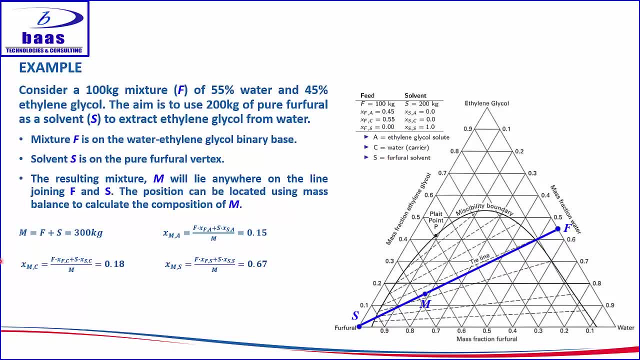 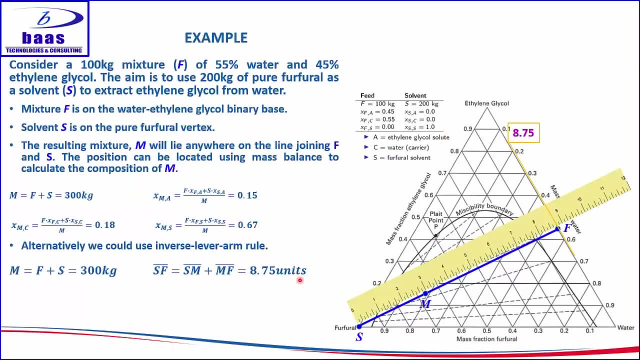 We need different specifications of F and S and then, as we have indicated here, we have calculated the composition and placed the location of M. Alternatively, we could use the inverse S app rules to locate M. The first thing we will do is: we will know. 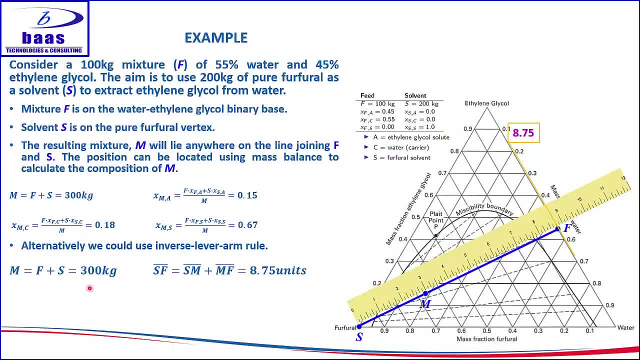 that the total mass of M will be that of F plus S, which is 300 kg, And then, as we have indicated in the previous slides, where we will see a movement point 옆, and then, as we have indicated in the previous slides, where we will see a movement point Start between F and S level greatest mass and total maximum mass and total maximum. 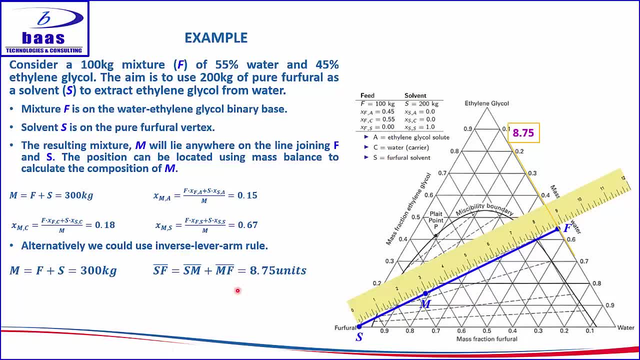 where we were reviewing the inverse lever arm rule, we know that SF, which is the total solution, will be the combination of SM and MF, and then, if we measure the length of this line segment, we find it to be 8.75 units, and this line is equivalent to 300 kilogram. we can look at using 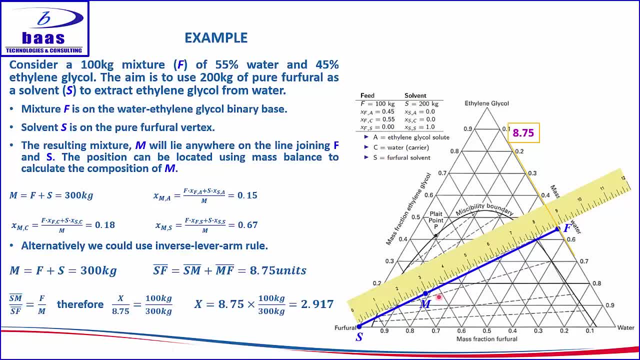 the, the lever arm rule, where we know that F will be donated by line segment SM and then M will be generated by line segment SF, which is the call the combined mixture, and then we have measured M to be 8.75 and then we can look for how long line segment SM will have to be so that we can 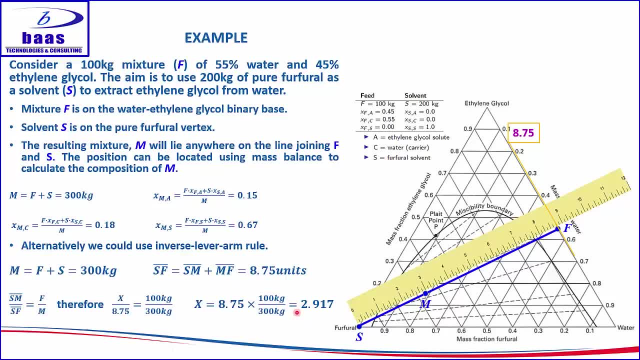 place it and calculating that, we find it to be 2.917. and if we look on our ruler here, it is indeed around there, just confirming that the lever arm rule in some way does agree with the calculations, as you can see that 2.917. 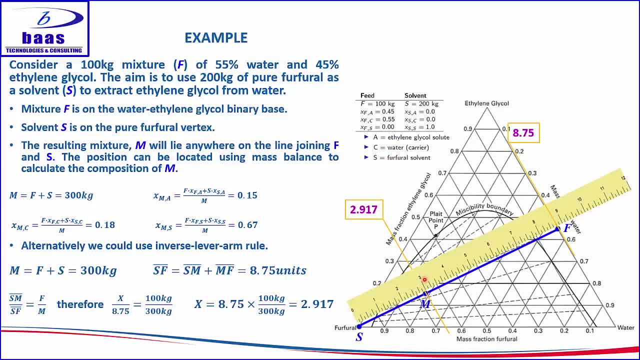 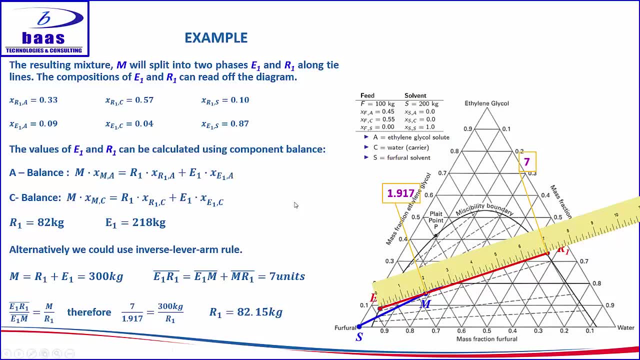 does pass through the point M, which we located, remember, using the composition space here. the resulting mixture M will split into two faces, E1 and R1, along the line segment SM and MF, and then we can look at the combination of M and MF and MF and. 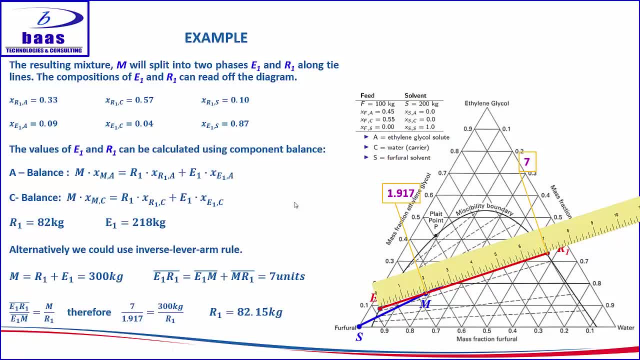 lines with with composition that can be rid of the miscibility boundary, which we have read here to be the values indicated here. we have read to be the values indicated here the values of E1 and our one, which are now the quantities, the kilogram quantities of E1 and R1, of the extract and the 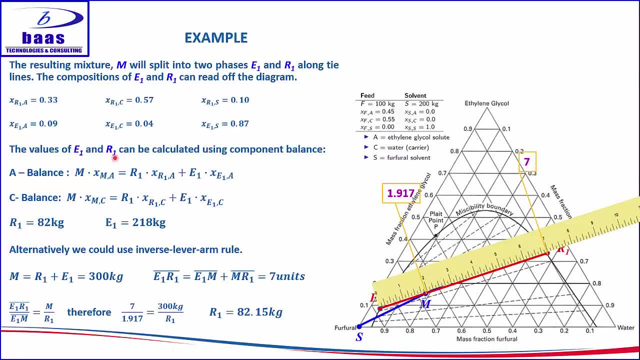 raffinate can be calculated using mass balance. here we can use composition space as we go around it. this much to be told in, and verses to know first. damn good, sisters. and that's all success so far. keep challenging your own. These�amandulationsong we can use for education classes during the classes, so that way you captured that part. so thank you. 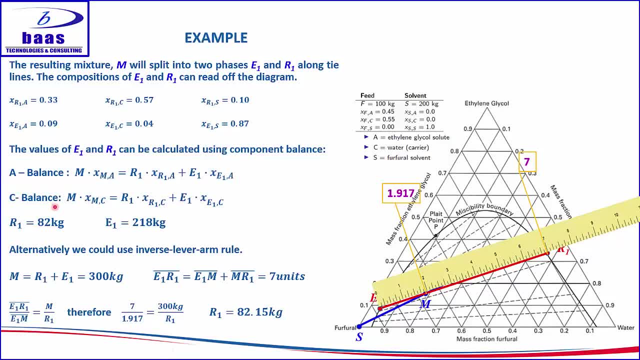 balance by doing component a balance and component C balance. looking at these two equations, the only two unknowns are that of r1 and e1, which are that of the quantities of the raffinate and the quantity of the extract. solving these two equations, for those two unknowns, we find r1 to be 82 kilogram and then e1. 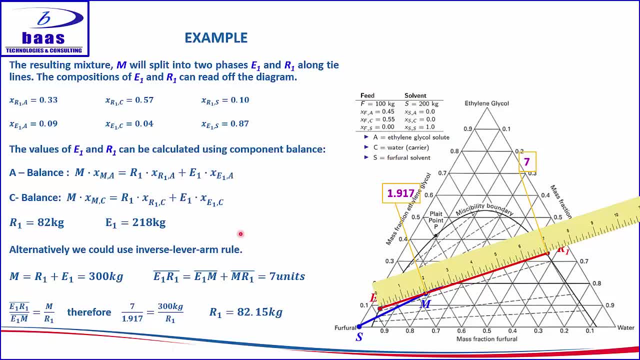 to be 218 kilogram. alternatively, we could have used the lever arm rule to calculate r1 and r1 and e1, where we will use a ruler to measure the line segments, we we can use the ruler to measure the length of length, segment e1.